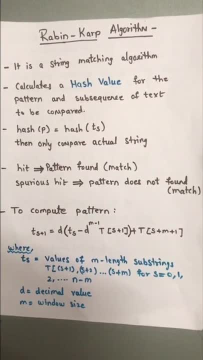 Hello everyone, I am Professor Akshata Rao, Computer Engineering Department, Viva Institute of Technology. In this video I am going to cover Rabin-Krapp String Matching Algorithm. In my previous video I have already covered two string matching algorithms. 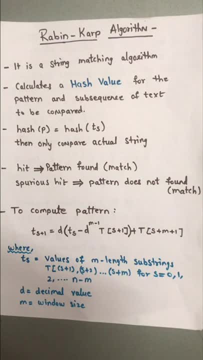 KNIFE String Matching Algorithm and KMP Algorithm. In KNIFE Algorithm we just compare text with the pattern with the help of window, And in KMP we use PyTable. In Rabin-Krapp Algorithm we can calculate hash value for the pattern and subsequence of the text to be compared. 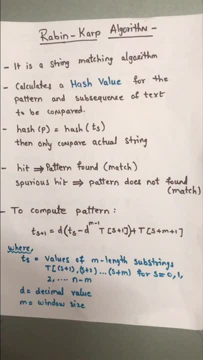 How to calculate hash value we will see later in this video. If the hash value of P is equal to hash value of TS, then only we can compare the actual string. If hash value does not match, then the algorithm will continue The hash value for the next subsequence. 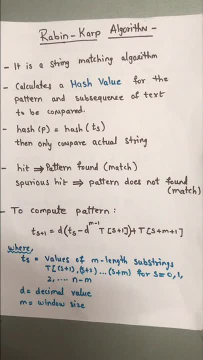 If the pattern is matched or pattern is found, then that time that thing is called as valid heat, Whereas if pattern does not match, then it is called as spurious heat. In this way there is only one comparison per text. subsequence and character matching is only needed when the hash values are matched. 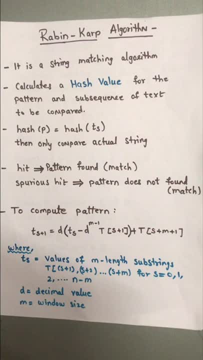 If hash values does not match with the pattern pattern's hash value, then we do not want to or we do not check the strings To compute a pattern. a pattern is given over here. TS plus 1 is equal to D, TS minus D raise to M minus 1.. 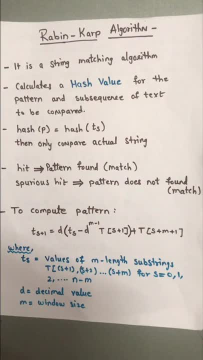 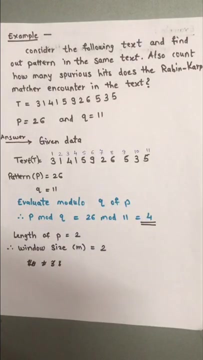 T of S plus 1 plus T of S plus 1.. M plus 1, where TS is the values of substrings and D is a decimal value. I will tell you what is decimal value and M is window size. Consider this example. 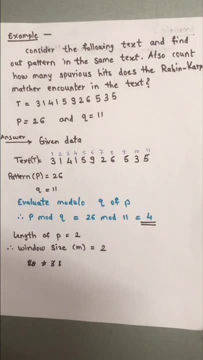 Consider the following text and find out pattern in the same text. Also count how many spurious heats does the Rabin-Karp matcher encounter in the text? Here the text is given and the pattern is given, and also Q is given. Now what is Q? 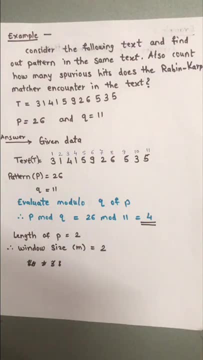 Q is nothing, but it is already given in the question. If it is not given, then consider Q's value as any prime number, any small prime number. Q is required to calculate mod, Mod is required to calculate hash values. So here given data is text. 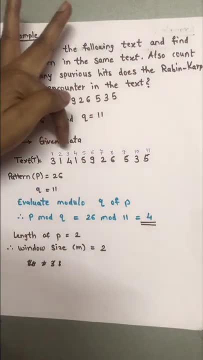 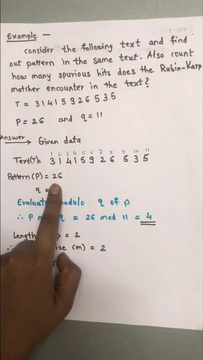 I have already written text over here and the indexes are given. Total 11 indexes are there. Pattern is 26.. Now we have to find out this 26 pattern. that is 2, 6 in the text above. Q is 11.. 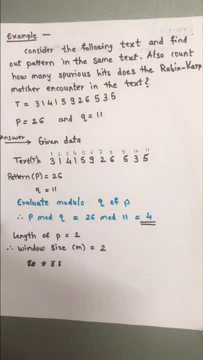 Now we can calculate: the modulo P mod Q, that is, 26 mod 11, is equal to 4.. Now we have to consider this 4 value as hash of P for the rest of the calculations And we will just check and consider this hash value with the remaining values. 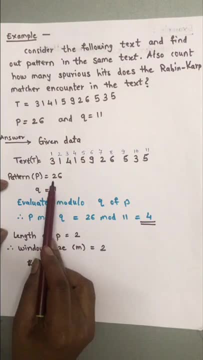 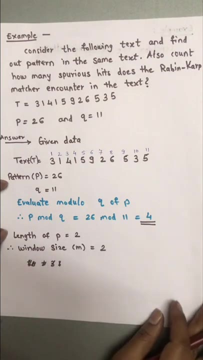 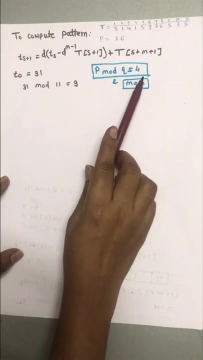 Length of the P is equal to 2. Because the exact values are 2.. Therefore, the size of M, or size of window, is also 2.. As I said, P mod Q was 4.- This I have already written over here- and M is equal to 2.. 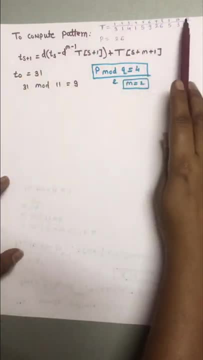 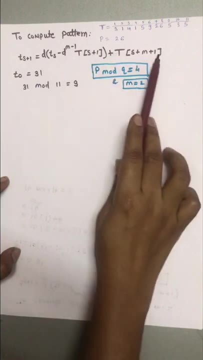 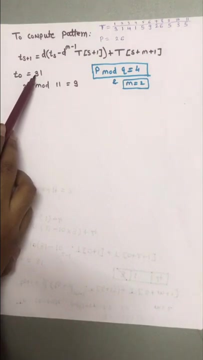 And the string it is written over here with the indexes P is equal to 26.. To compute the pattern, I have written the formula over here In the first iteration, that is T0, we will consider index 1 and 2, that is 31.. 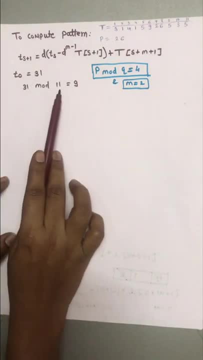 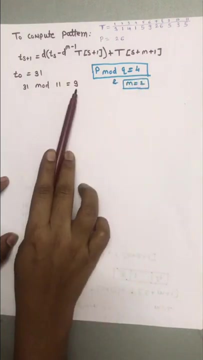 So 31.. If we mod 31 with 11, we will find out that the value of hash of TS is equal to 9.. Now consider: hash of P is equal to hash of TS. 4 is not equal to 9.. 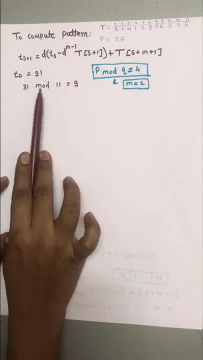 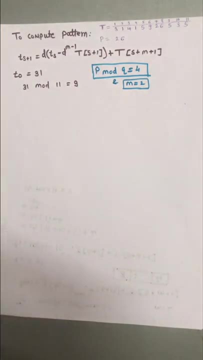 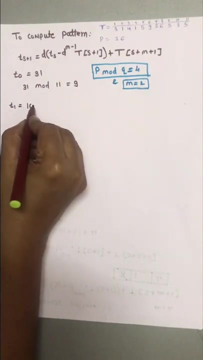 Therefore MAC does not found. That means we don't have to cross check the pattern with the text. Just calculate the next value Now: T1.. T1 is equal to D. D- I am writing as 10.. As I said, D can be any value. 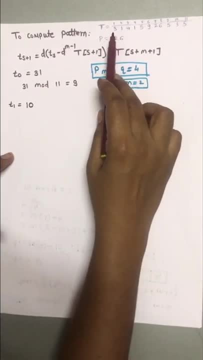 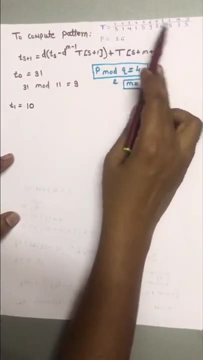 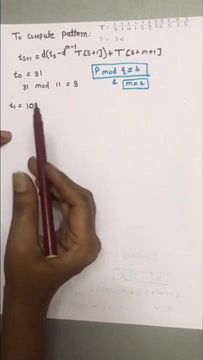 But now we can see here, these values are from 0 to 9.. These values are from 0 to 9. So this is nothing but decimal value. So I am considering these values as 10.. Then TS. 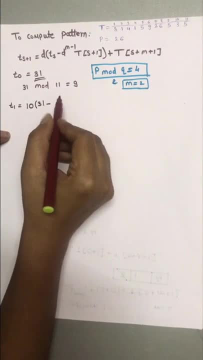 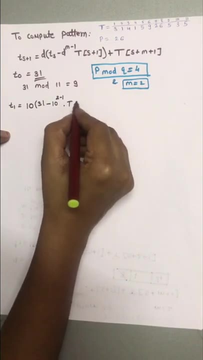 TS is 31 minus 10. raise to 2 minus 1. Because M is equal to 2.. 10 into T of S plus 1.. S is nothing but value of sub sequence And it starts with 0. So consider 0 first. 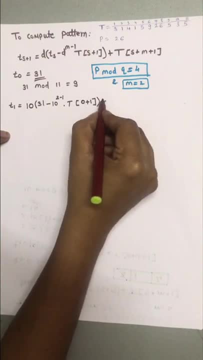 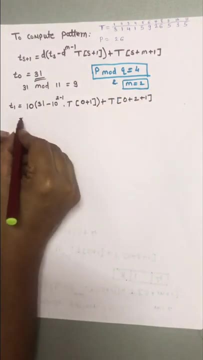 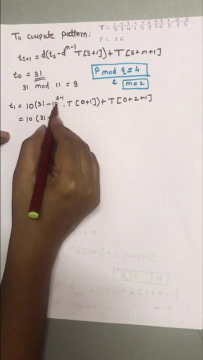 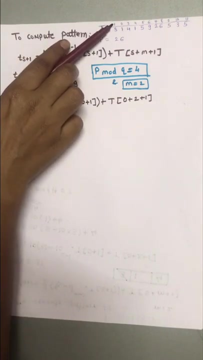 Then 0 plus 1 plus T of 0 plus 2 plus 1. 10 into 31 minus 10, raise to 1. 1, that is 10 into t of 1. so t of 1, that is index index 1. we have to check index index. 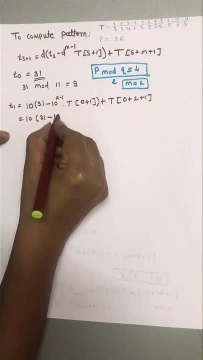 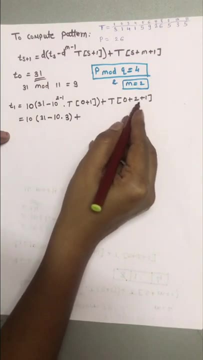 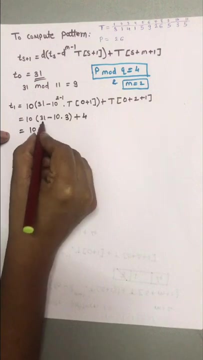 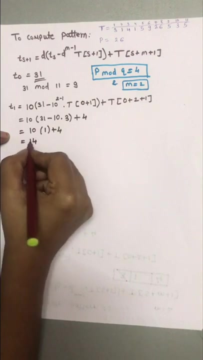 1 is 3. consider 3. so 10 into 3 plus t of 3. t of 3 is 4. the value is 10. 31 minus 30 is 1 plus 4. final answer is 14. so next subsequence is 14. so this why I am calculating this, because 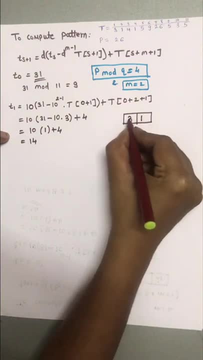 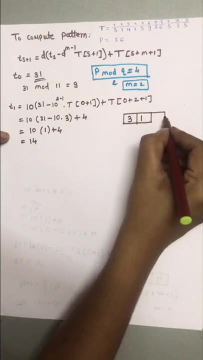 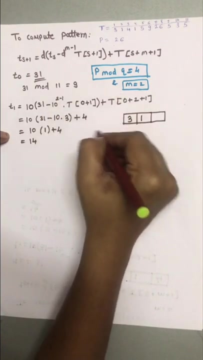 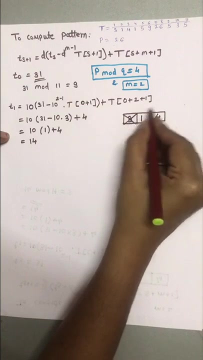 the previous text was 31. it is not matching with the pattern 26, so now I have to calculate the next subsequence. what will be the next value? so for this I have calculating entire thing. So next value is 14. because the size of window is 2, we have to discard this value and we 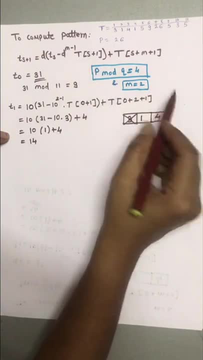 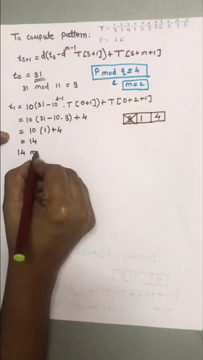 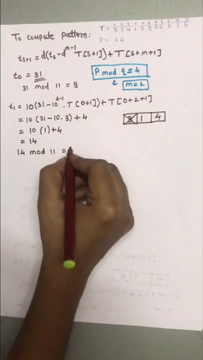 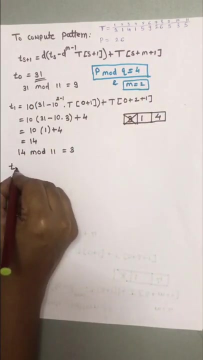 have to compare this value with the pattern. that is 14 with the pattern. it is not matching with the pattern, right? so take hash value: 14 mod 11 is 3,. 3 is not matching with the pattern, So we will write as 4, then calculate t2 10. now the new ts value, that is 14 minus 10 raise. 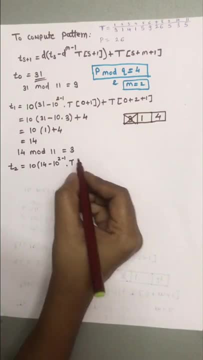 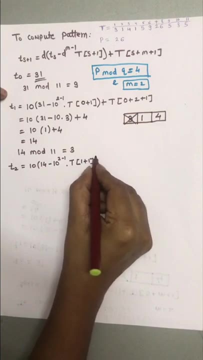 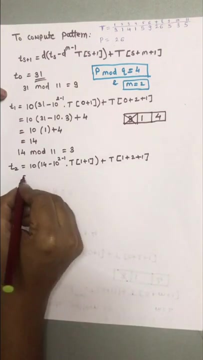 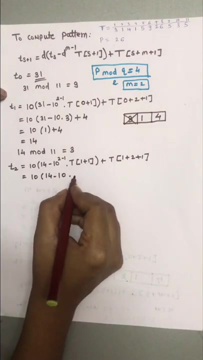 to 2 minus 1 into t. now the value of ts plus 1 will be 1 plus 1 plus t into 1 plus 2 plus 1.. equal to 10, 14 minus 10 into t of 2, t of 2 is 1, here t of 2 is 1, we have to check. 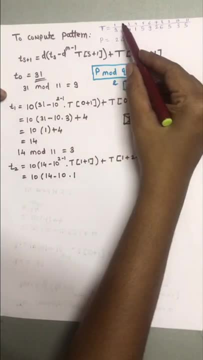 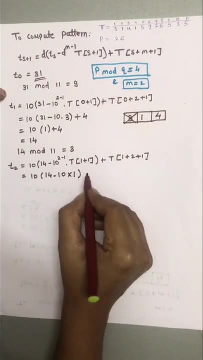 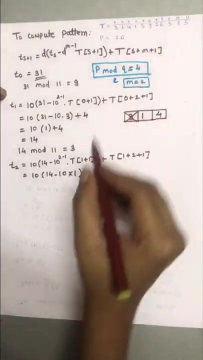 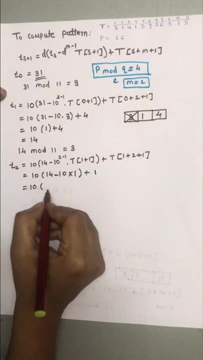 the index, not the value. t of 2 is index 2 and considering this value as 1, so this is multiplied t of 4, t of 4 is also 1, so it is 1, now 10, 14 minus 10 is 4 plus 1 equal. 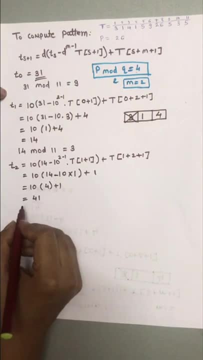 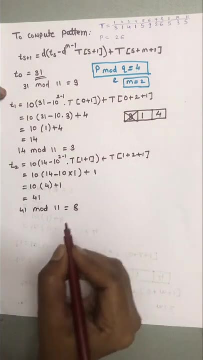 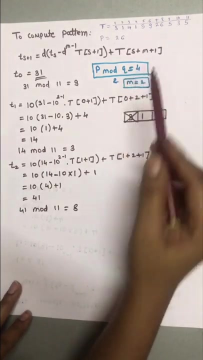 to 41, now 41 mod 11,. 41 mod 11 is 8,. now we have to check the index, not the value. t of 2 is index 2 and considering this value as 1, we have to check the hash value with t. hash value 8 is not matching with 4, next, 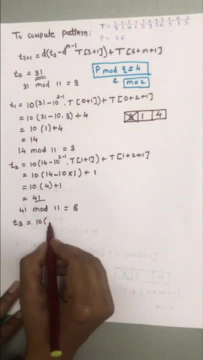 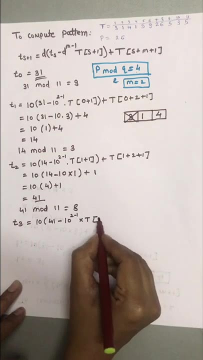 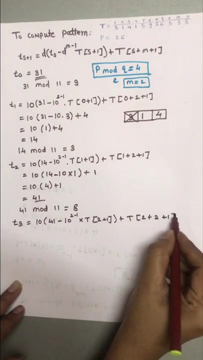 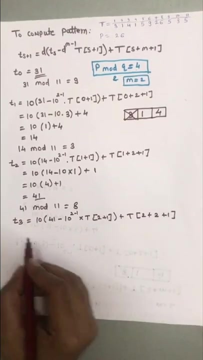 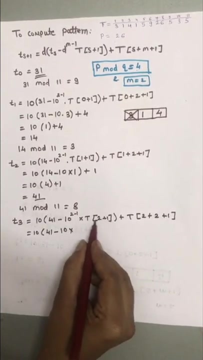 iteration 10. new value for t1 minus 10: raise to 2 minus 1 into t of 2 plus 1 plus t of 2 plus 2 plus 1.. This is new value. This is value of windows and this is the formula now: 10, 41 minus 10 into t of 3, t of 3 is: 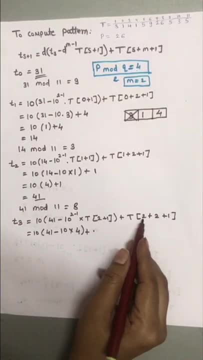 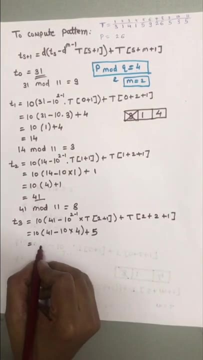 4 plus t of 5, t of 5 is 5, so the final value is t. this is 41 minus 40 is 1 plus 4 is 1,. 5 is equal to 15, now check value. hash value: 15 mod 11, value is 4, now check value of. 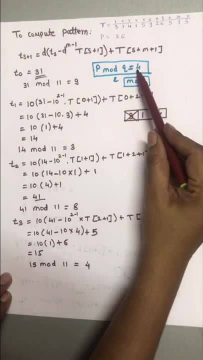 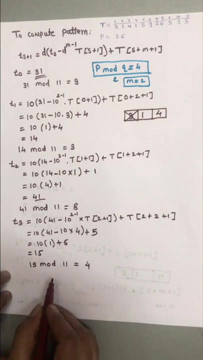 hash hash value of t is with hash value of t it is matching. 4 is equal to 4, so we have to check the string. what is the string? 1, 5.. 1, 5.. 1, 5.. 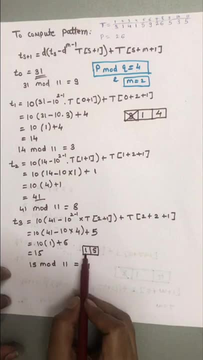 So here it is 1, 5, now we are considering window as 1, 5 and the pattern we are searching for is 26,. it is not matching with the actual pattern. that, because 2 is not equal to 1,. 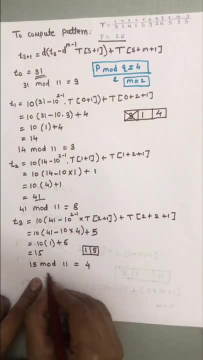 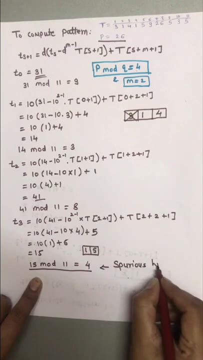 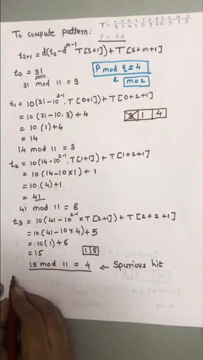 so it is not matching. that means this heat is nothing but spurious heat. spurious heat. Now we will consider, Now we will consider the next iteration: t4,. t4 is equal to 10, again the same formula. 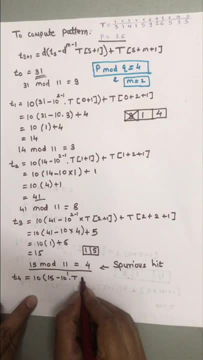 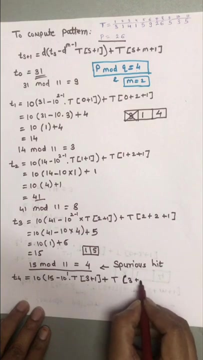 15 minus 10 raise to 1 into t of 3 plus 1, we have considered in the previous iteration t of s plus 1. value is equal to 2, now it is 3 plus t, 3 plus 2 plus 1, t of s plus 1,. 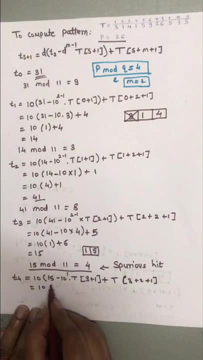 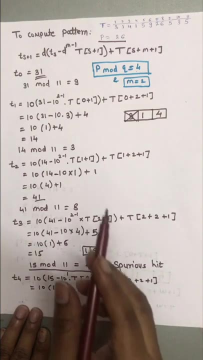 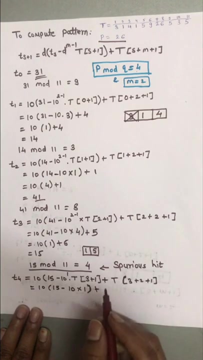 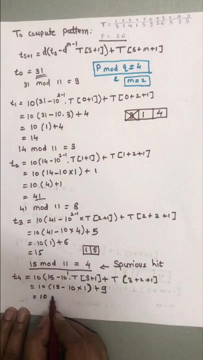 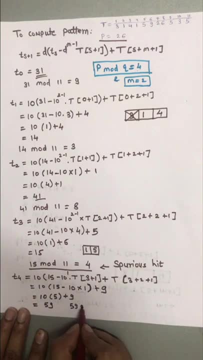 So it is 1 plus 3, this is 6, t of 6 is 9 and the final answer is t of- sorry- 10 in bracket 5 plus 9, equal to 9.. Now 59 mod 11 is equal to 4.. 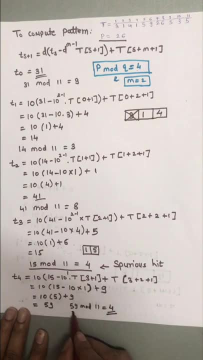 Again, this value is matching with the p value. So we have to check again, check this pattern with the original pattern. Original pattern is 26 and this pattern is 59.. 2 is not matching with 5.. That means this hit. 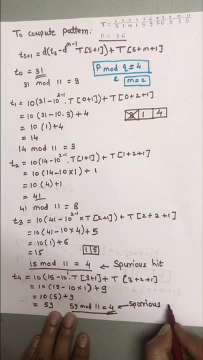 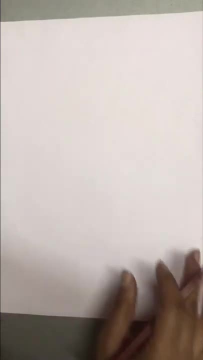 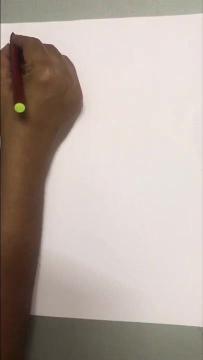 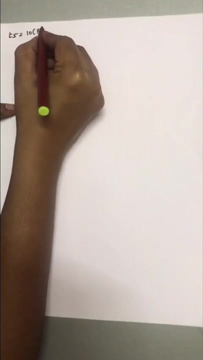 Is again spurious hit. So now t4, we have to calculate t4.. Sorry, we have already considered t4.. Now it is t5.. t5 is 10 in bracket. In previous iteration we have got the value of t4 as 59.. 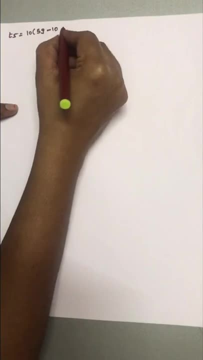 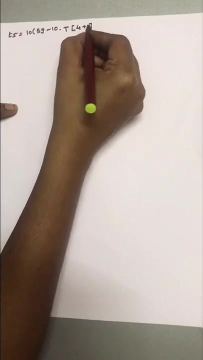 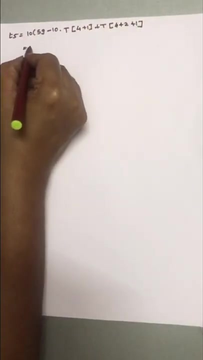 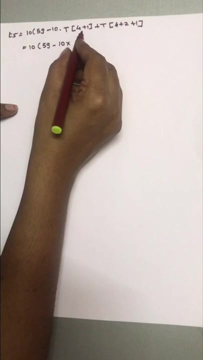 So 59 minus 10 into t in bracket 4 plus 1 plus t of 4 plus 2 plus 1 equal to 10, 59 minus 10 into t of 4 plus 1.. 4 plus 1 means index of 5.. 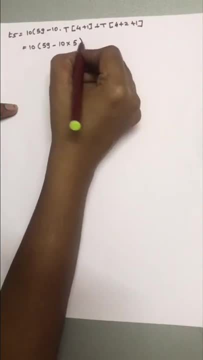 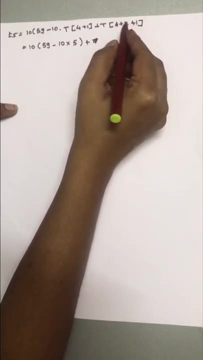 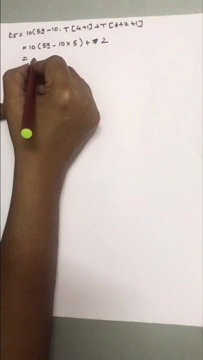 Index of 5 is 5 plus t- sorry t, not t- 4 plus 2 plus 1 is 7.. t of 7 is 2.. So, considering 2 and the final answer is 92.. 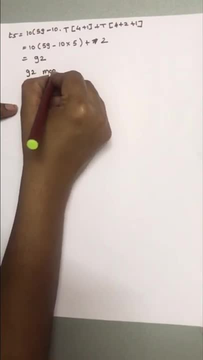 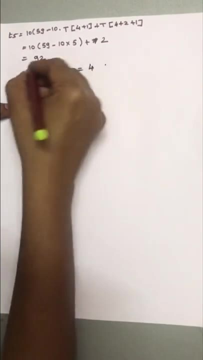 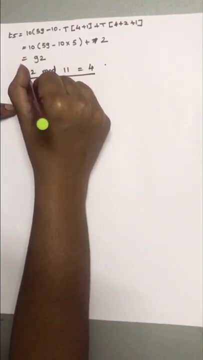 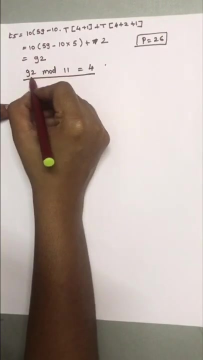 So 92 mod 11 is equal to 4.. So we have to consider this iteration And we have to compare pattern with the newly found find out string substring. So pattern was p was 26 and the value is 92.. 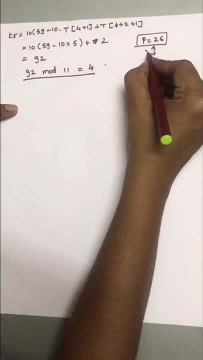 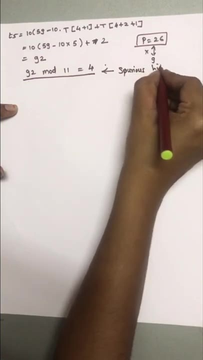 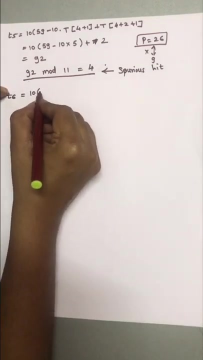 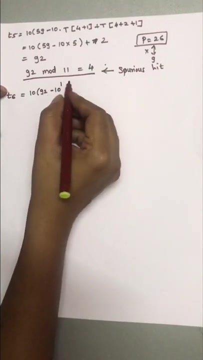 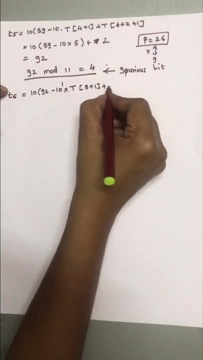 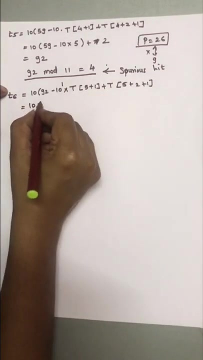 9 is not matching with 2.. So it is nothing but spurious. hit Next iteration t6.. t6. t6 is 10 into 92 minus 10, raised to 2 minus 1.. That is 10 raised to 1 into t of 5 plus 1 plus t of 5 plus 2 plus 1, equal to 10 of 92 minus. 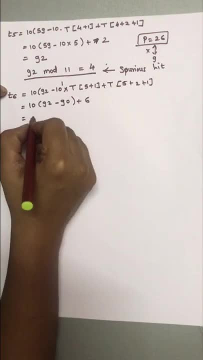 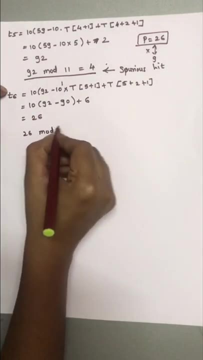 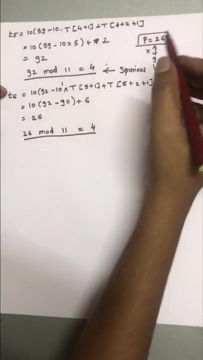 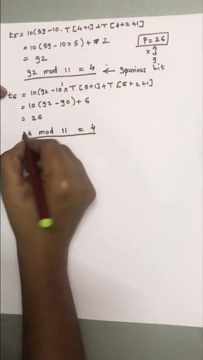 6 and we got value as 26. now we have to check 26 mod 11. value is 4 again. we got value as 4 and the previous hash value was 4. now check with the pattern. actual pattern 2 is matching with 2. 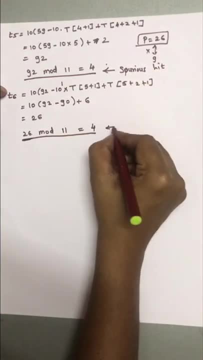 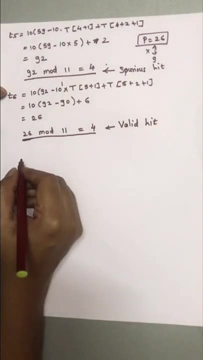 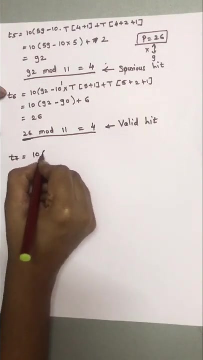 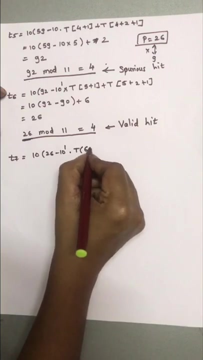 6 is matching with 6, so at this point we got valid hit. so this is valid hit again. continue with the same process. t7 is equal to 10 in bracket 26 minus 10. raise to 1 into t of 6 plus 1. 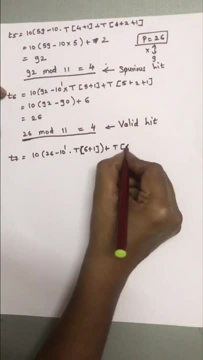 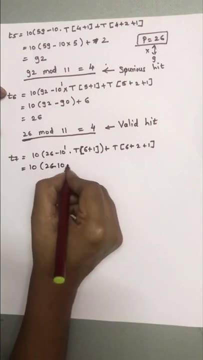 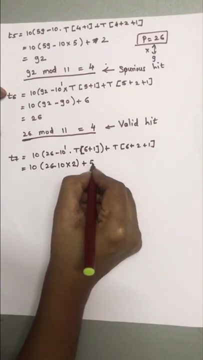 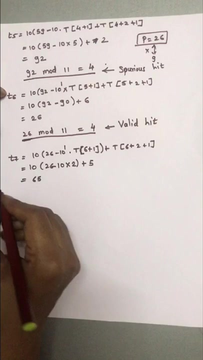 plus t of 6 plus t of 6 plus 1. 2 plus 1 is equal to 10. 26 minus 10 into 2 plus this is 5 equal to 65. so 65 mod 11 is equal to 10. 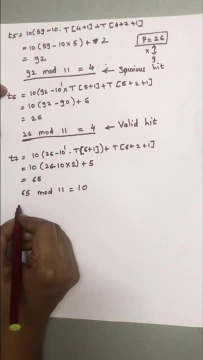 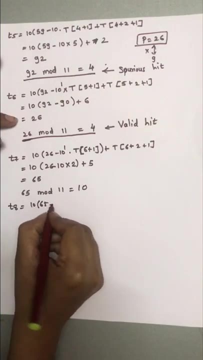 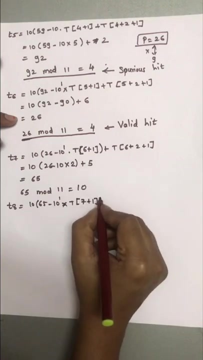 10 is not matching with the actual value of hash p, that is 4. so consider next iteration: 10 of 65 minus 10 raise to 1 into t of 7 plus 1 plus t of 7 plus 2 plus 1. 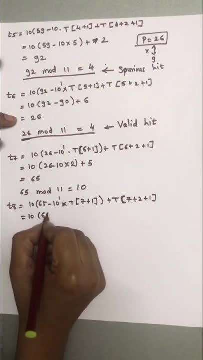 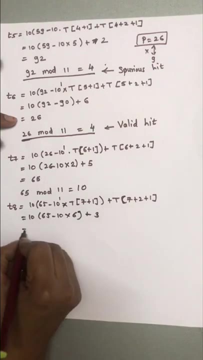 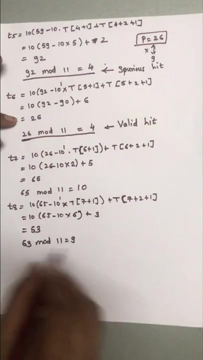 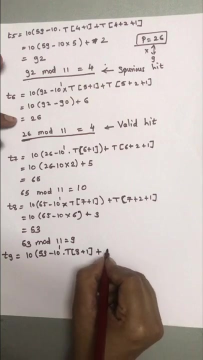 equal to 10, 65 minus 10 into 6 plus 3, equal to 53. 53 mod 11 is equal to 9. it is not matching with the original pattern. so next, 10 53 minus 10 raise to 1 into t, 8 plus 1 plus t, 8 plus 2 plus 1. 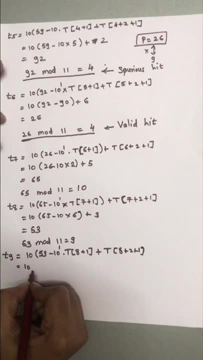